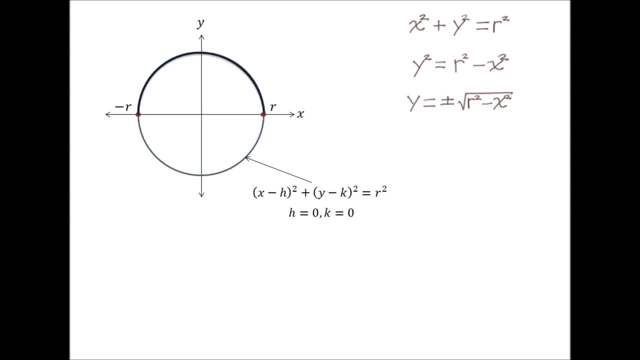 x squared. However, we are only concerned for the positive side, as that is the function of our semicircle and that will be the function to be revolved. so we let f of x just equal radical of r squared minus x squared. 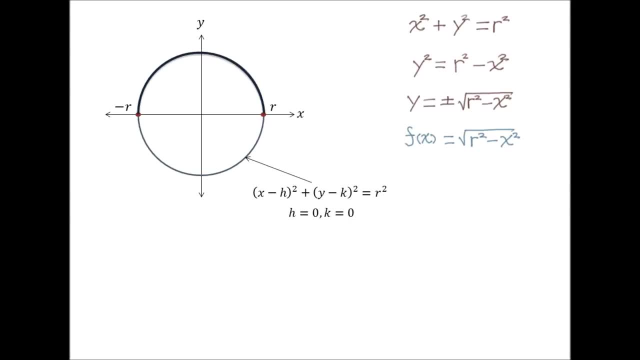 Now that we have set up our graph and equation, we are ready to start with our method. But before I jump to the disk method as a quick side help for those of you who struggle understanding this method, you know that if we take an instantaneous strip of length f of x and a width dx, having an instantaneous area da, 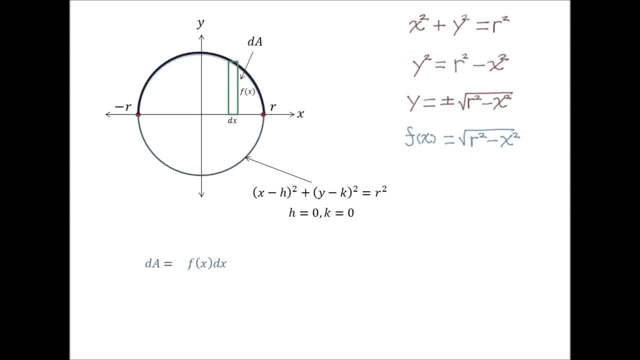 where da equals f of x, dx, and integrate from x equals negative r all the way to x equals r. we will simply just get the area under the curve f of x or the area of the semicircle, But now in the disk method, instead of an instantaneous rectangular strip. 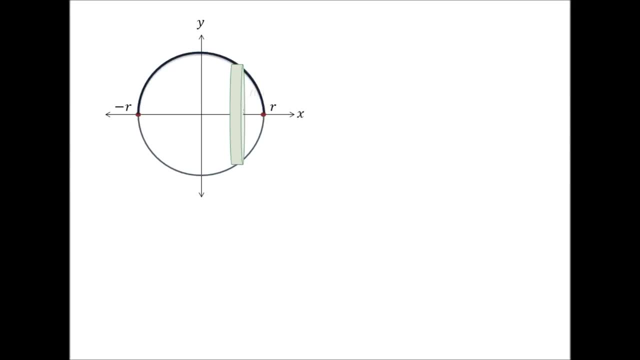 we now take an instantaneous cylindrical disk of radius f of x and height dx, with its instantaneous volume dv equal to pi times f of x squared times dx, because the volume of a cylinder is pi times height times radius squared, And integrating this from negative r to r, we will then get the volume of our sphere. 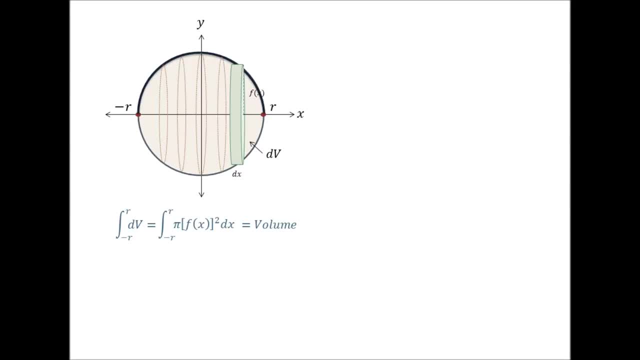 And now that we have our integral, we plug in for f of x and we get the volume equal to the integral from negative r to r of pi times the radical r squared minus x squared squared dx. Seeing that the square and the radical cancel and that we can pull the constant pi out, we then get the following: 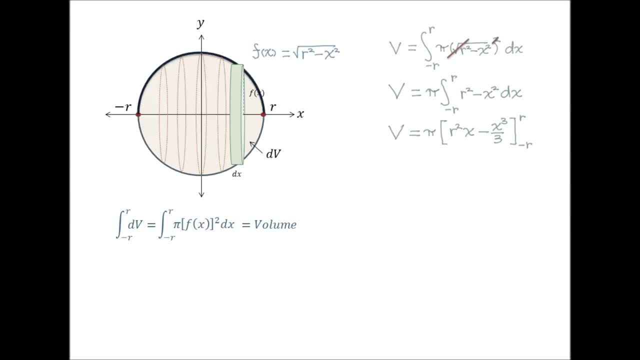 And now we integrate the integral and we get the quantity r squared x minus x cubed over 3 from r to negative r, Plugging in our limits. we then get the following: Distributing the negative in r squared times, negative r and negative times, the quantity negative r cubed over 3,. 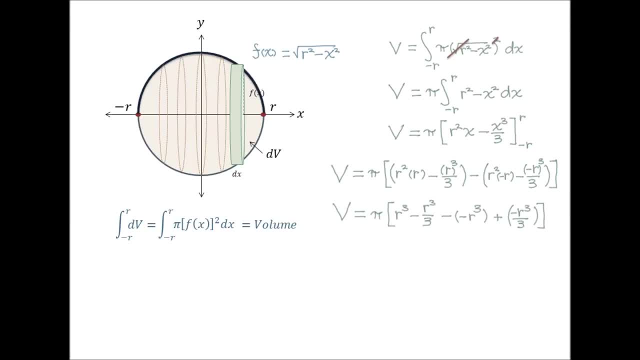 we then get volume plus r cubed over 3, plus r cubed over 3.. And seeing r cubed minus negative r cubed is 2r cubed and that negative r cubed over 3, minus r cubed over 3,.